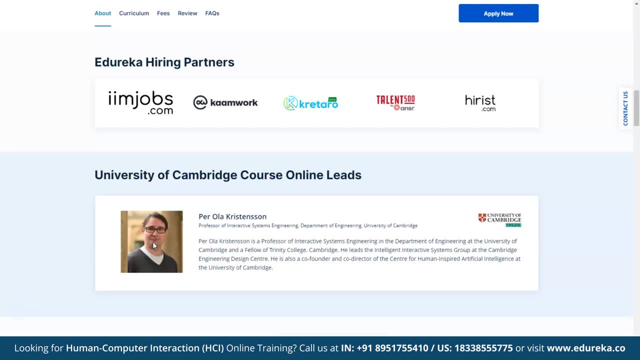 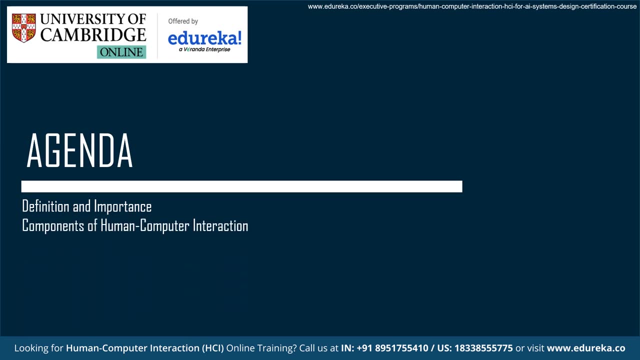 please see the course link provided in the description box below. In this video we will cover the definition and importance of HCI, along with the components of human-computer interaction. We'll also discuss the factors in HCI, the HCI design processes, the human-computer interaction in different industries. 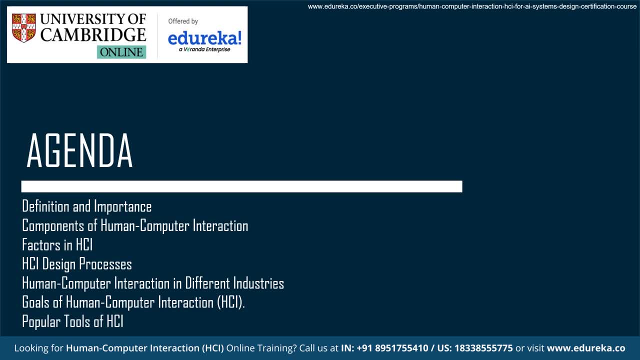 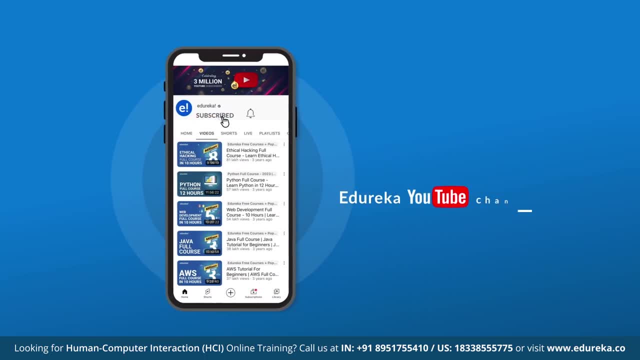 of human-computer interaction. Finally, we will also discuss popular tools of PCI. But before we get started with the topic, please consider subscribing to our YouTube channel and hitting the bell icon to stay updated on the latest tech content by Edureka Also. 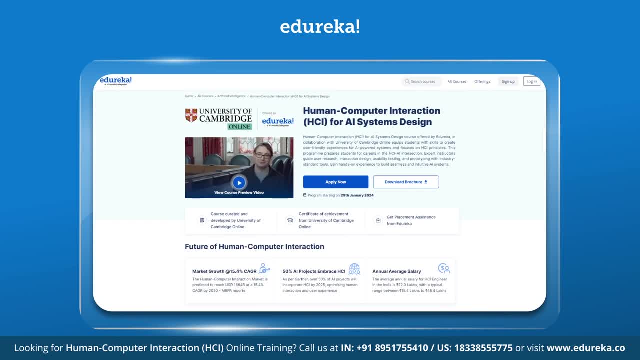 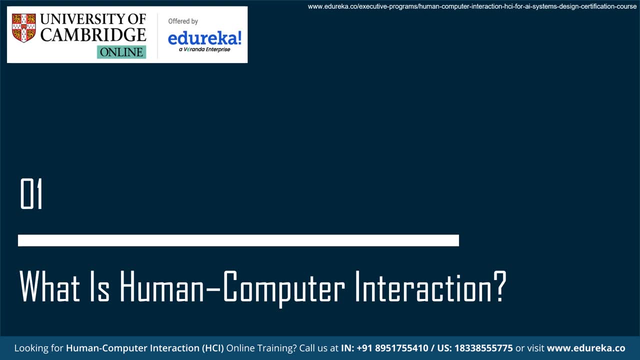 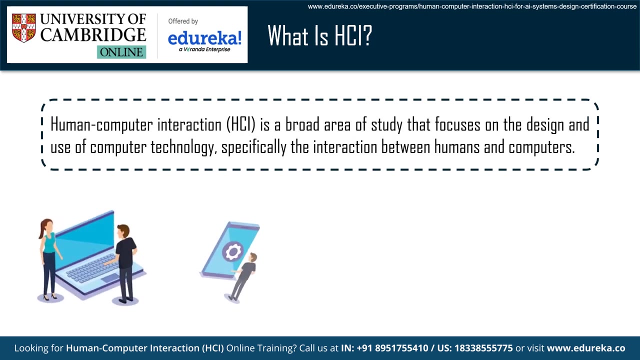 visit the Edureka website for training and certification courses. The link is in the description box below. Let's see what PCI is and why it's important in improving our technological experiences. Human-computer is a broad area of study that focuses on the design and use of. 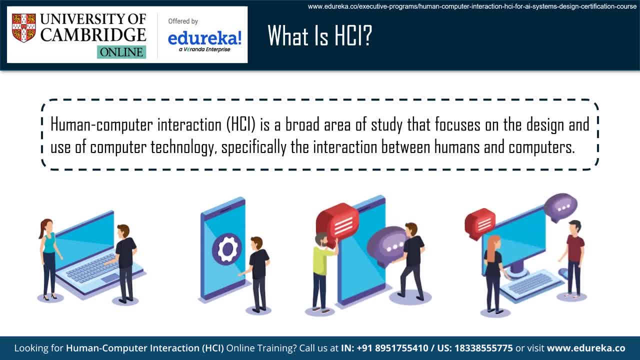 computer technology, specifically the interaction between humans and computers. It investigates how people interact with computers and the extent to which computers are developed for successful interaction with humans. HCI researchers observe human interactions with computers and design technologies that allow for normal human-computer interactions. 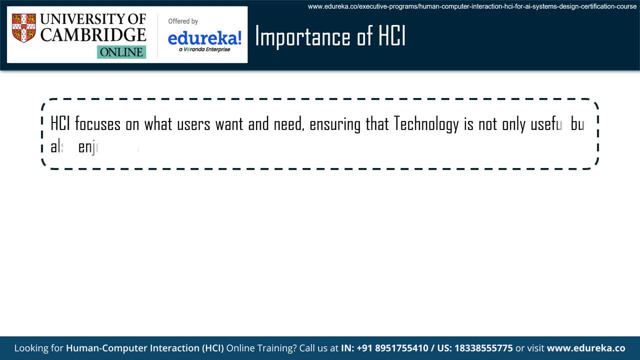 Importance of PCI. PCI, which stands for human-computer interaction, plays an important role because it helps make gadgets and software easy to use for everyone, regardless of experience levels. It's like making things that people understand. PCI focuses on what users want and need, ensuring that technology is not only useful. 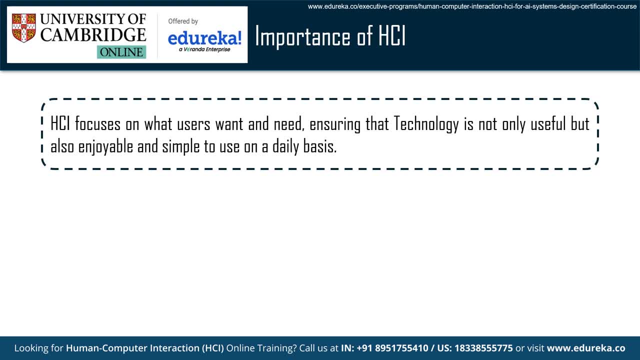 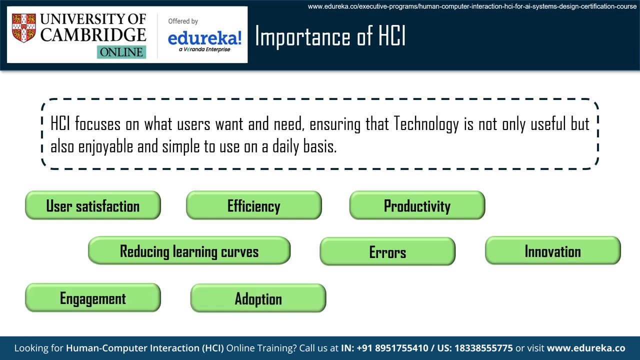 but also enjoyable and simple to use on a daily basis. Such as PCI, enhances user satisfaction, efficiency and productivity, while reducing learning curves and errors. It encourages innovation, engagement and adoption, providing companies with a competitive advantage. Ethical considerations in HCI ensure responsible and trustworthy technology. 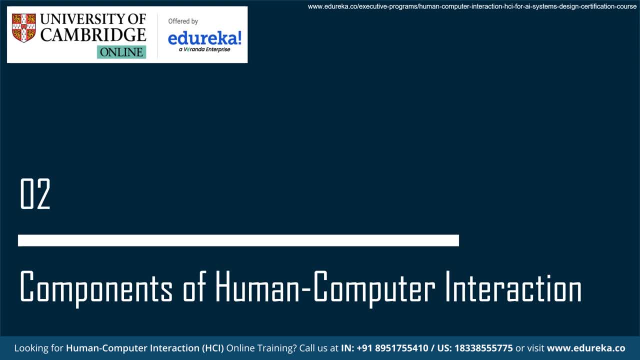 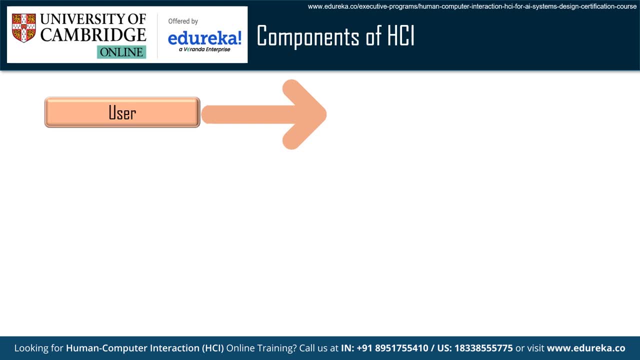 Components of human-computer interaction. Human-computer interaction is made up of four key components: User – individuals or groups participating in a shared task, each bringing their own set of needs, preferences and behaviors to their interaction. Task with a specific goal. 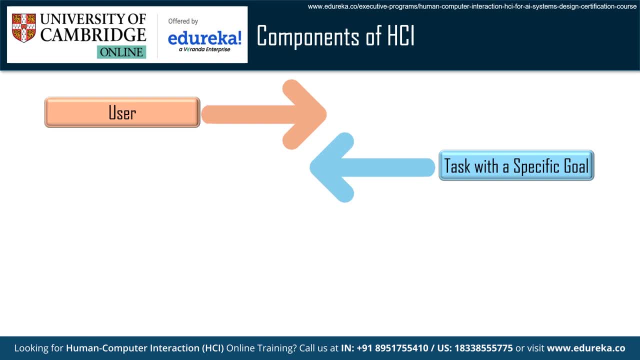 Users interact with a computer system with specific goals in mind, which drive their actions and interactions. Interface – the tools and platform that facilitate user-computer interaction, including design elements and input-output methods. Context – the context in which the interaction occurs, influencing user behavior and system design considerations. 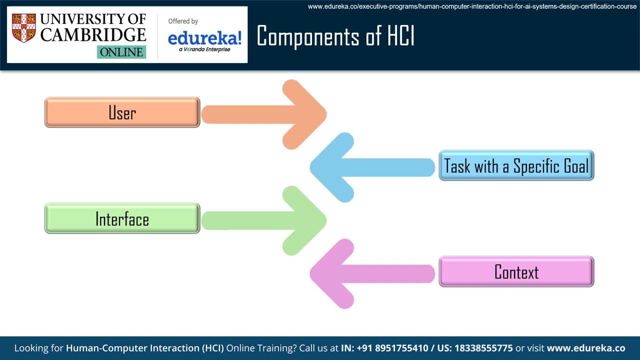 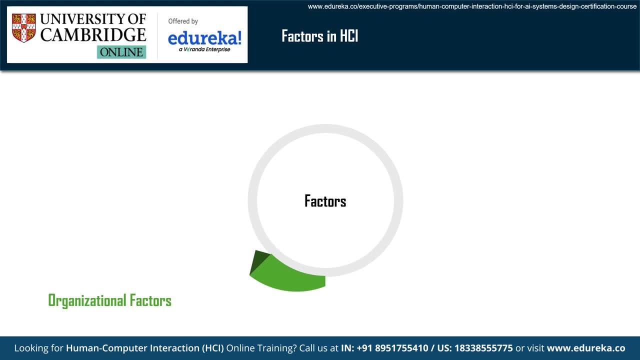 Physical surroundings, technological environment and social aspects are all part of the context Factors in HCI. Organizational factors – training, job design, politics, roles and work organization are vital organizational factors influencing HCI. Environmental factors – environmental considerations, such as noise, heating. 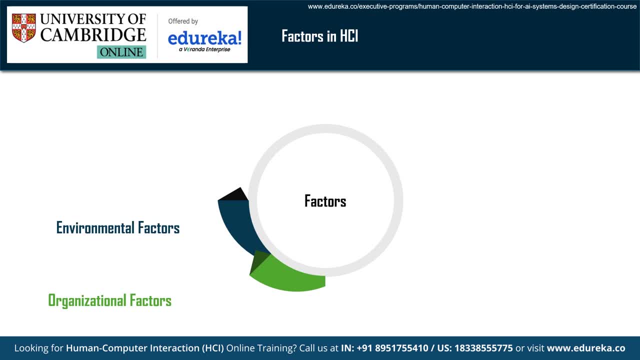 lighting and ventilation impact the user experience. Health and safety factors play a crucial role in ensuring the well-being and safety of users. User-related factors include cognitive processes, motivation, enjoyment, satisfaction, personality and experience. Comfort factors encompass aspects like seating. 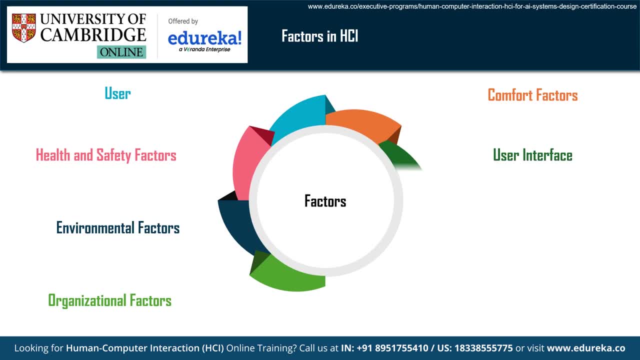 equipment and layout for optimal user comfort. User interface considerations involve input and output devices, dialogue structures, color usage, icons, commands, navigation graphics, naturalize language, user support and multimedia. Task factors include complexity, novelty, allocation, monitoring, user skills and impact system design. Productivity factors aim to 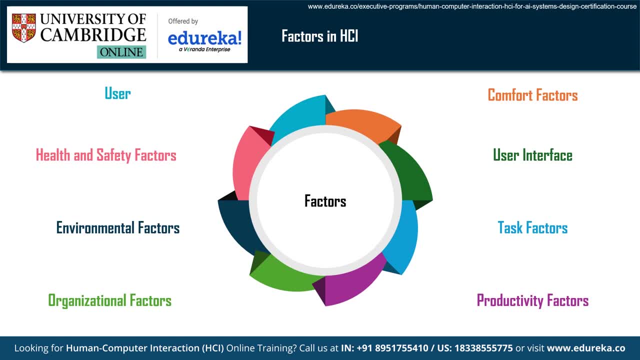 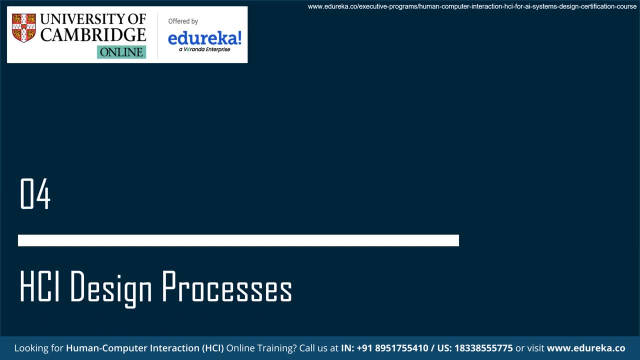 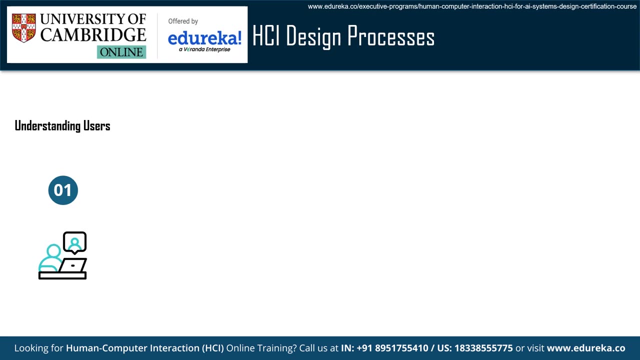 increase output quality and innovation while decreasing costs and errors in system design. HCI Design Process. HCI Design Process is an integrated approach that includes understanding users. Understand user needs, behaviors and preferences. research and analysis. task and requirement analysis, identify and analyze specific tasks. 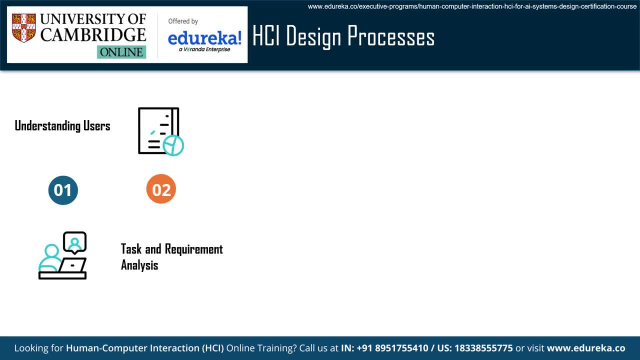 that users must complete, collecting both functional and non-functional requirements. conceptualization and prototyping: create interactive prototypes for visualizing and refining the user interface and develop high level design concepts. usability testing: evaluate prototypes with real users, identifying problems and refining the design for maximum usability. detailed interface design and implementation: create a detailed user interface design taking. 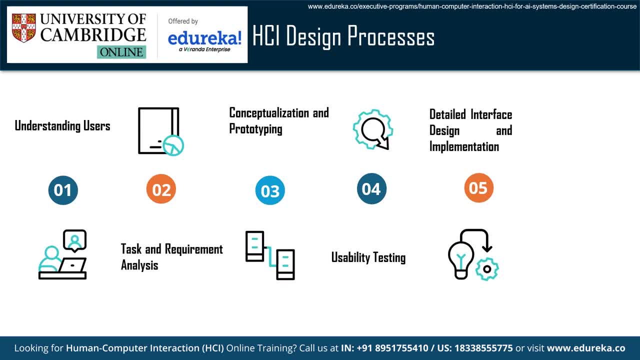 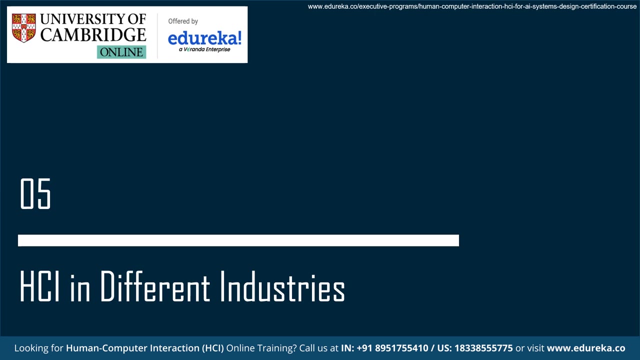 layout, navigation and visual elements into account and then implement the system based on the finalized design. evaluation, deployment and maintenance. perform additional usability testing, deploy the system and continuously monitor user feedback and support system performance. human computer interaction in different industries. here are few ways human computer interaction affects various industries. healthcare: hci ensures that medical devices and 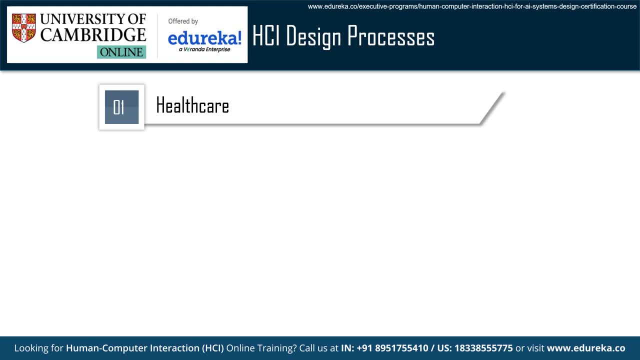 electronic health records have user-friendly interfaces, improving interactions between healthcare professionals and patients. finance: hci influences the design of online banking platforms and trading interfaces in the finance sector, improving user experience for financial transactions. education: human computer interaction plays an important role in educational technology, influencing the design of e-learning platforms and interactive educational. 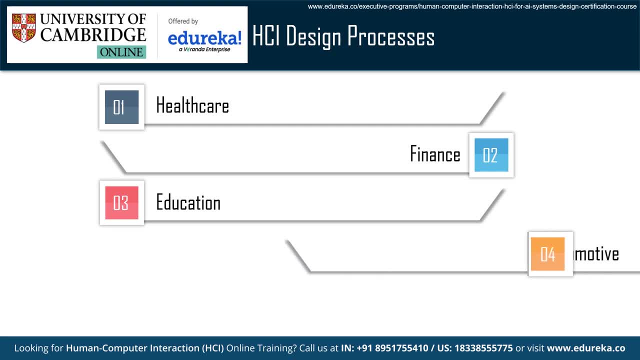 tools for effective learning experiences. automated hci has been seen in the design of in-car interfaces and voice recognition systems in the automotive industry, enhancing safety and usability for drivers and passengers. entertainment: human computer interaction principles are used in the entertainment industry, influencing the design of video game interfaces and streaming services. goals of human computer interaction usability: 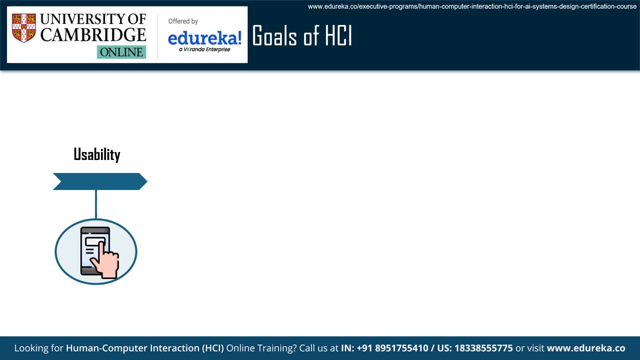 make sure that technological interfaces offer a positive user experience, are simple to use and are easy to learn. user-centered design. throughout the design process, give the needs and preferences of the user top priority in order to create interfaces that live up to your needs, user expectations, efficiency. create user interfaces that maximize productivity and workflow. 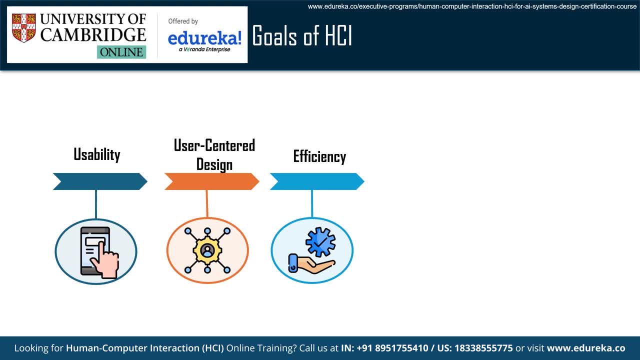 by enabling users to complete tasks fast and with little effort. accessibility: make sure that people with different abilities can use technology, as this encourages inclusivity and equitable access to data and services. user satisfaction: make an effort to design user interfaces that not only fulfill functional specifications but also enhance the user's emotional experience, which will increase user.